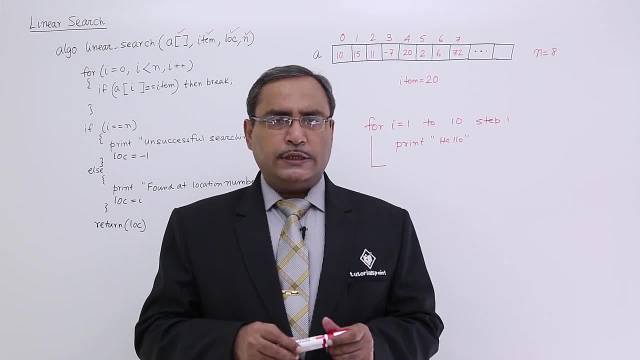 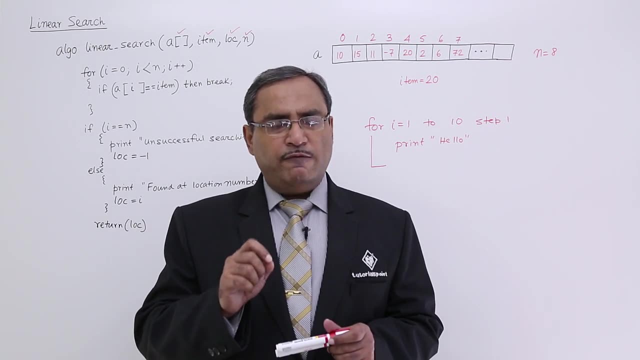 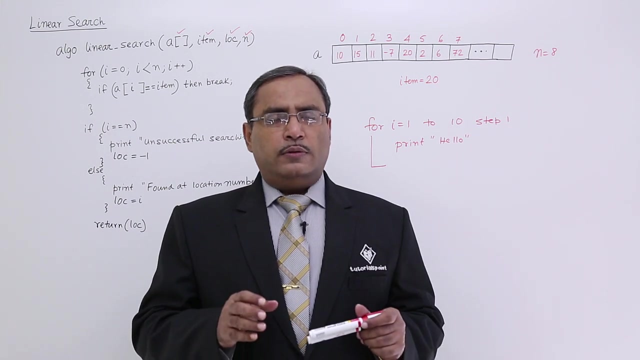 of data. So here the worst case complexity will be n and the best case complexity will be 1, because I can find that particular item at the very first location of the array, and the average case complexity will be n by 2.. Now let us discuss this one with some proper algorithm and example. Let us suppose I am having 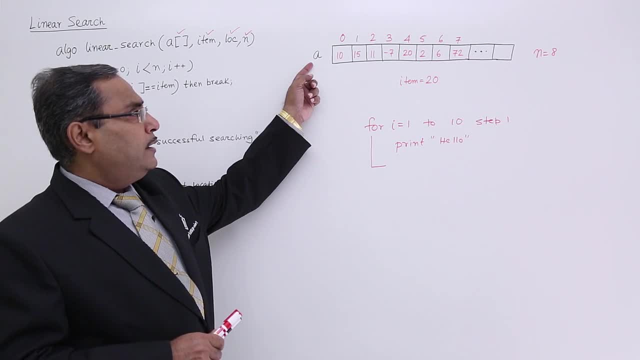 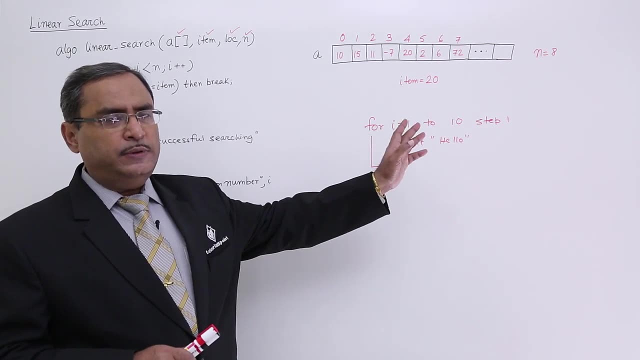 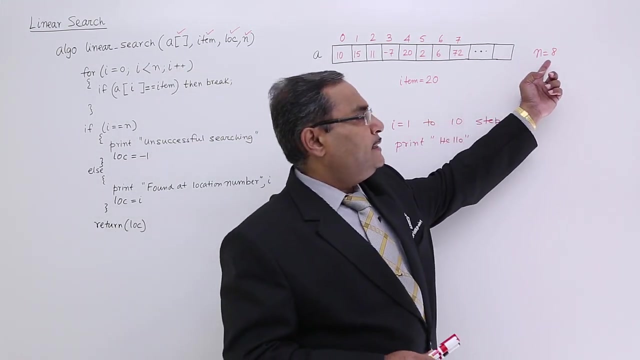 one array with the name a and which is having, say, 8 valid data, and obviously I need not to bother that. what is the max lock? what is the size of the array? because I shall confine my searching operation within 0 to n minus 1 location. Here the value of n is equal to 8, so 0 to 7.. So let 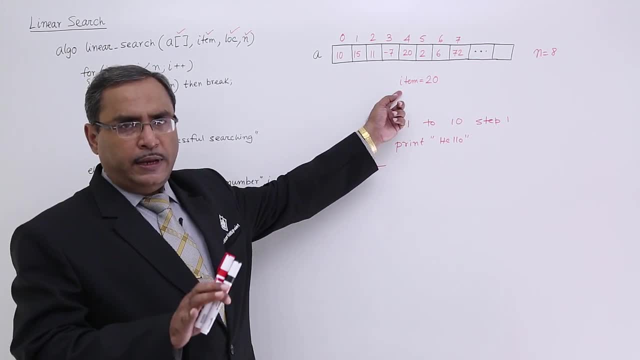 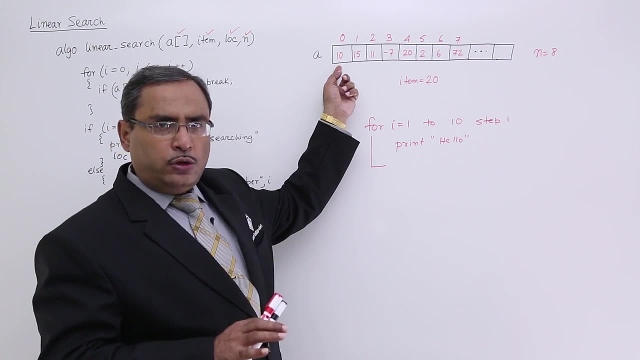 us suppose I am searching for the item which is equal to 20 for the time being. just consider. So at first I shall match 20 with this particular location's content, which is 10, and they are not equal. then I shall go for the next location. 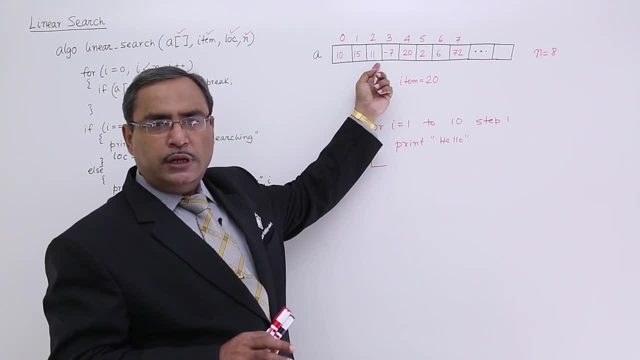 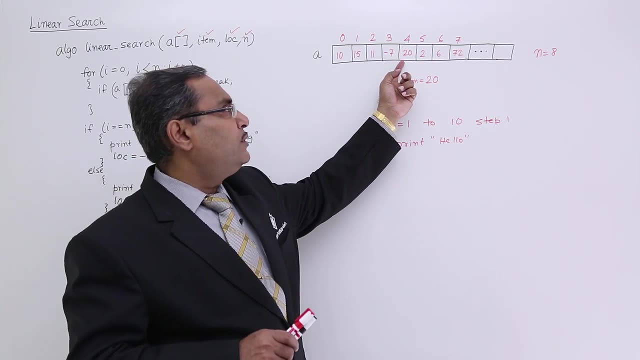 15, 20. they are not equal, then I shall go for the next location: 11, 20. they are not equal, then I shall go for the next location: Minus 7, 20. they are not equal, then I shall go for the next location: 20 and 20. they are matching with each other. In that case, I shall 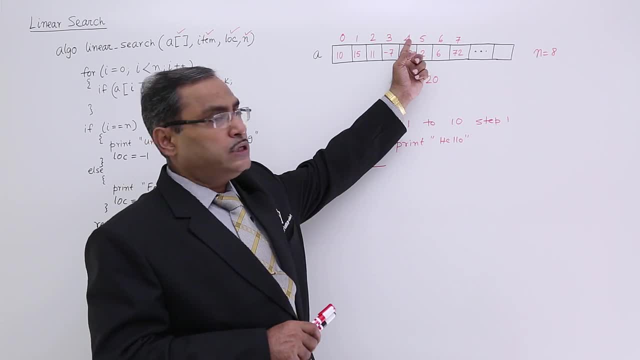 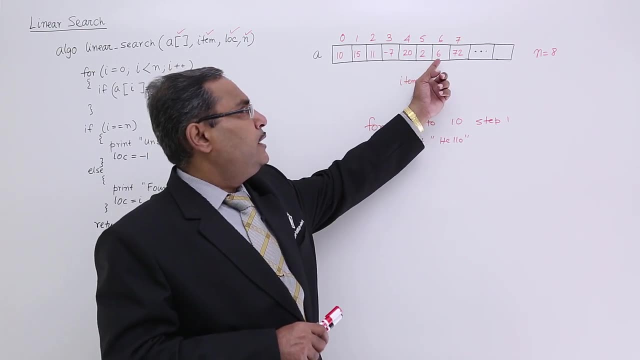 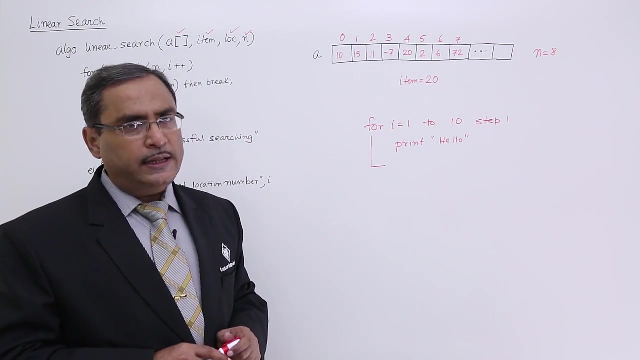 print the successful searching and also I shall return the location number, that is my 4.. So in this way, if it is 200, then I shall go on searching and I shall terminate at that very particular place where I am comparing it with the last data available in the array. 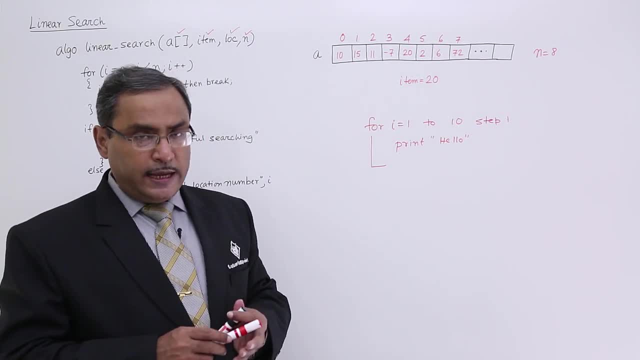 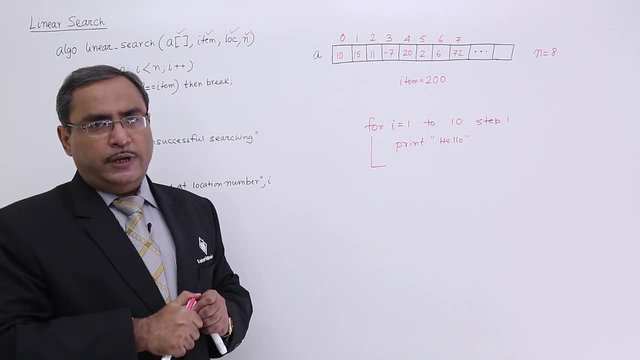 So then in that case I shall print unsuccessful searching if my searching item is not 20 but 200.. Ok, so in this way the searching will be done. so that is why it is called linear search or sequential search. Now I want to mention one thing about linear search Now. I want to mention one thing about linear search. I want to mention one thing about linear search. This is called linear search. So this is called linear search. So this is called linear search. So you can just jump on or you can come out anywhere in the search field, even if I want. 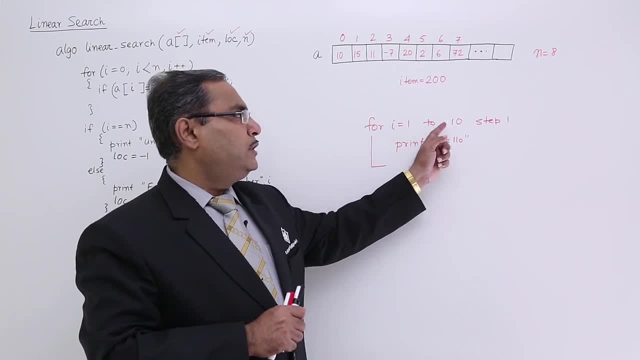 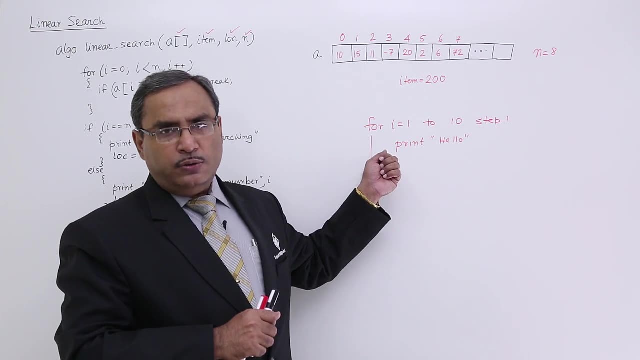 to have some information to search, interesting, сохранized And for me. I know my 김 seguro, And if you want to grown something, to check something, I can count two hundred, że one hundred that is just equal to one hundred seven, so you can find middle one, anything. 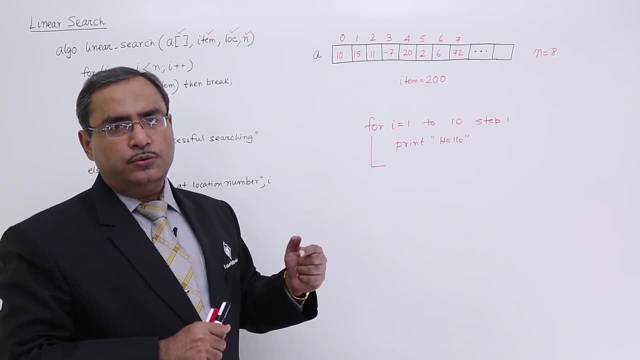 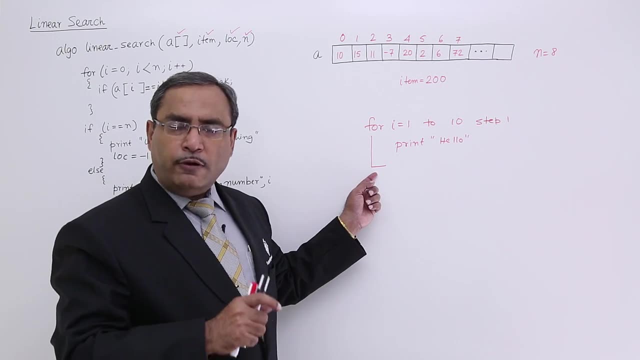 you want, But in real world, because of, Because of, Because temple event events, andrahina events, It is also. No, this is basically something I cannot take into account, But just like this, So you see, here there has was a extra number like this zero that was saved from. 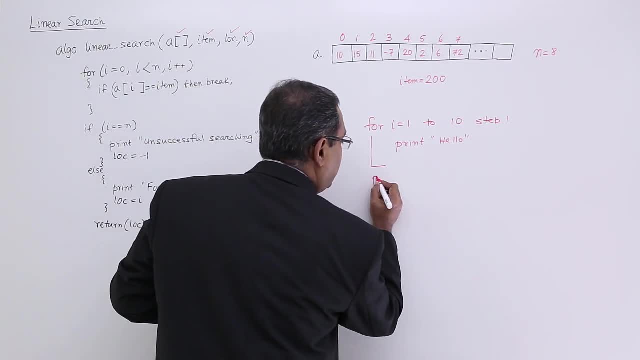 zero. Let us see, let us find this first one indice, all right. and the problem again is this: we were getting these two Nowсти. now we are going to look at the next news formula, that if I write print, if I write print after this particular loop, then what will be the? value of i is getting printed. my answer is here. the value of i will be 11. always remember this one. so because 1 to 10, so i will be ranging from 1 to 10 and loop will get executed. after that the value of i will become 10 plus 1, that is 11, and 11 is not within this limit. 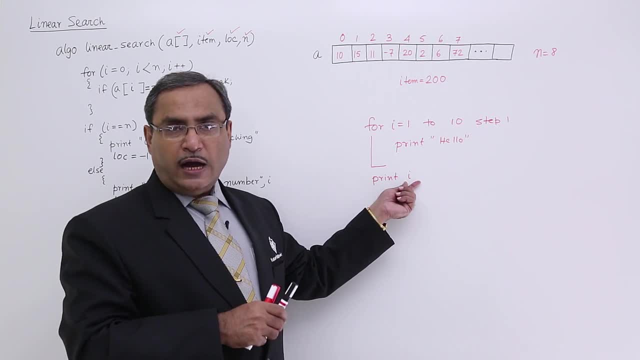 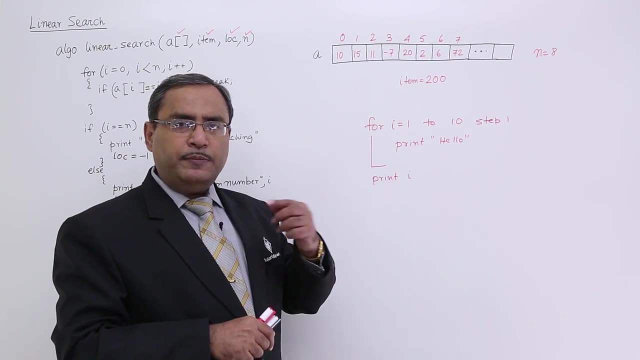 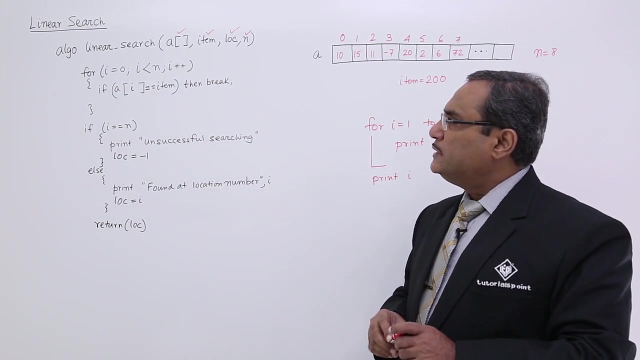 so it will come out from the loop. but the value of i, if you print after coming out from the loop, it will print the value 11. so this 11 value in i. this concept I have used in my linear search algorithm, so this is my algorithm. the name of the algorithm is algorithm linear. 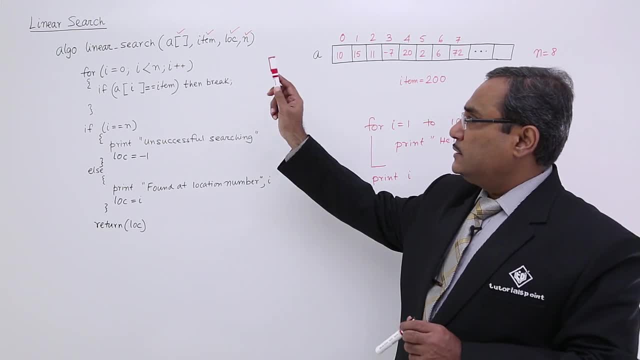 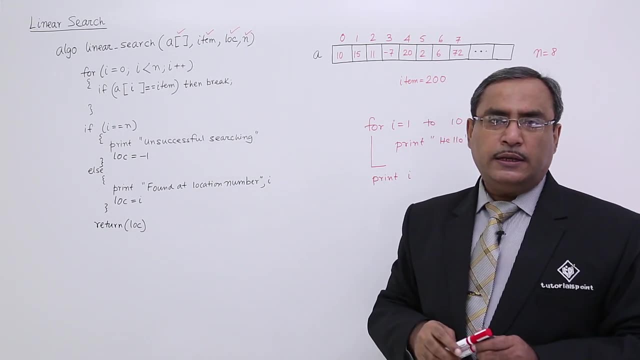 search. here I am passing 4 parameters: 1, 2, 3, 4. the first parameter is the name of the array. the second parameter is my item element, The third parameter is the lock and last parameter is n. a means the name of the array. 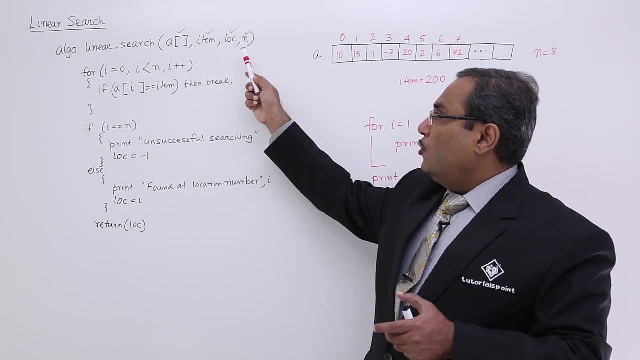 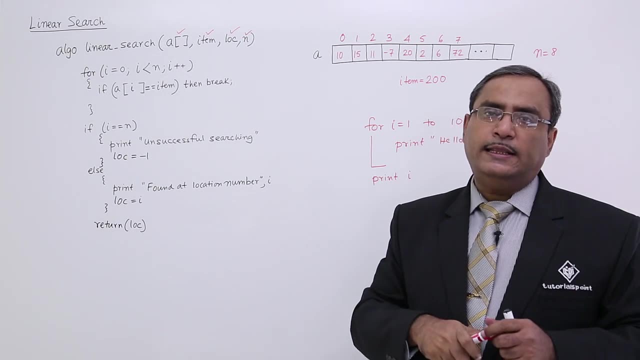 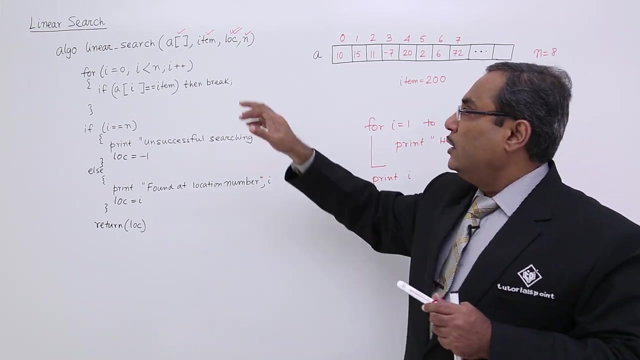 item means the value which has to be searched, and lock means at which location I am getting this particular item, and this n is the number of data residing in the array. ok, now, this lock is my output argument, so I am putting double tick there only to indicate that lock. 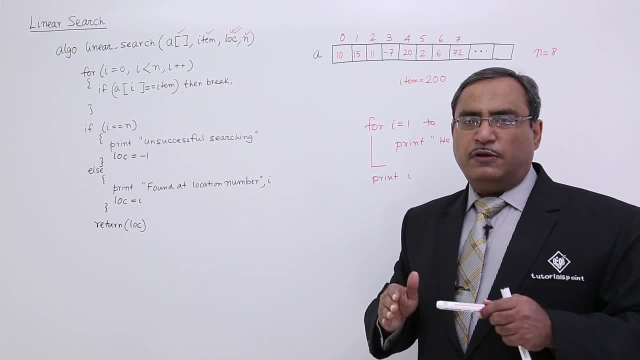 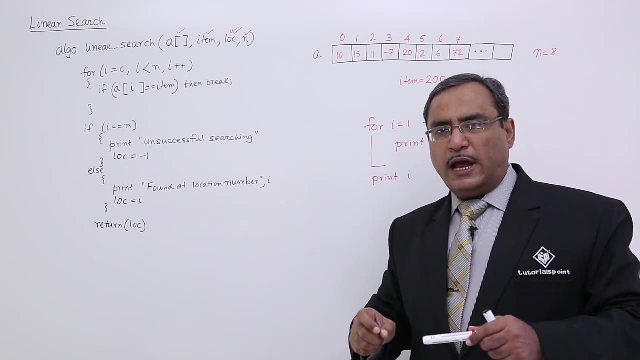 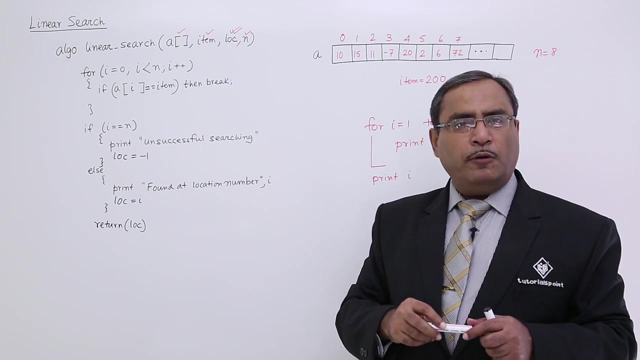 is my output argument. if the lock value is any one of the values in between 0 to n minus 1. That means successful searching has been done and the data item has been found at the location lock. but if the return value of lock is minus 1, that will indicate unsuccessful searching. 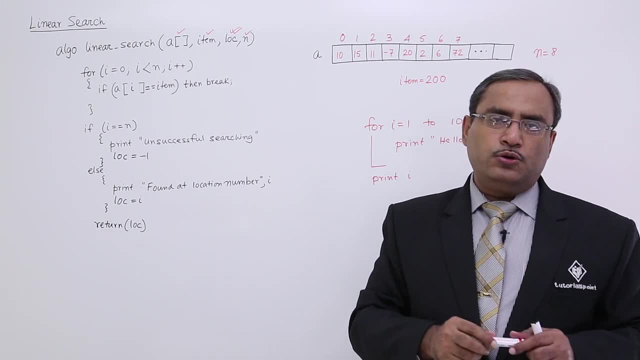 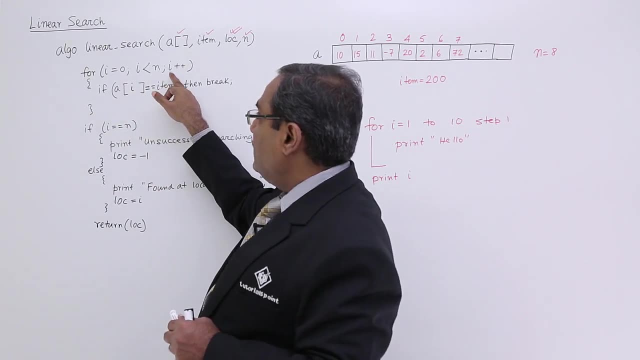 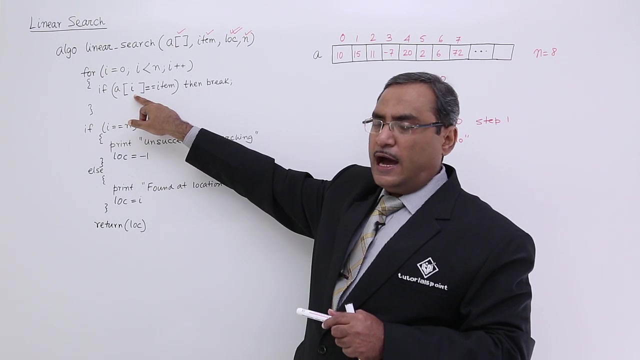 of the item within the locations 0 to n minus 1 of the array. so for: i is equal to 0, i less than n, i plus plus. if ai is equal to item, that means I am searching for item in each and every location of this array a. 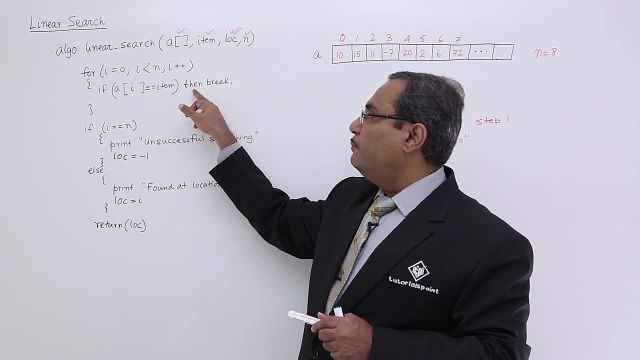 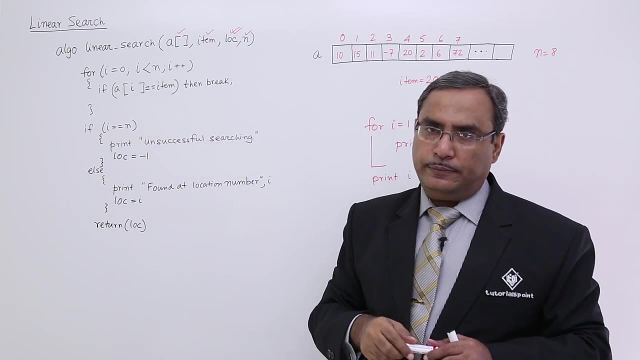 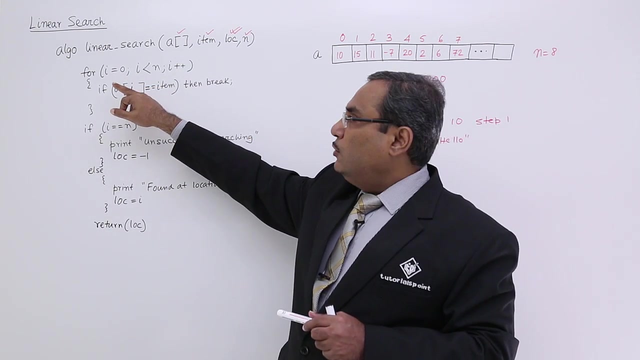 If I am finding this one matching, then break. break will come out. break will just make the control come out from the for loop, otherwise this loop will go on executing. ok, So please use this concept and tell me what will be the value of i if the loop gets executed.